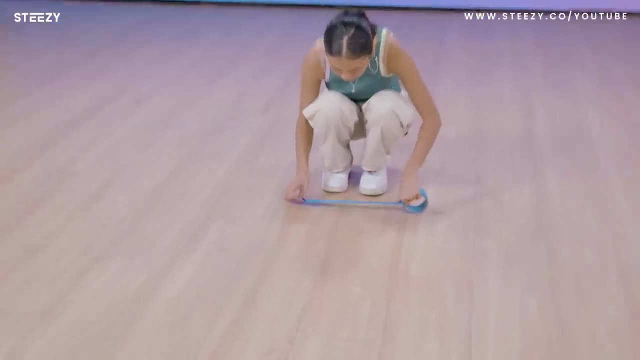 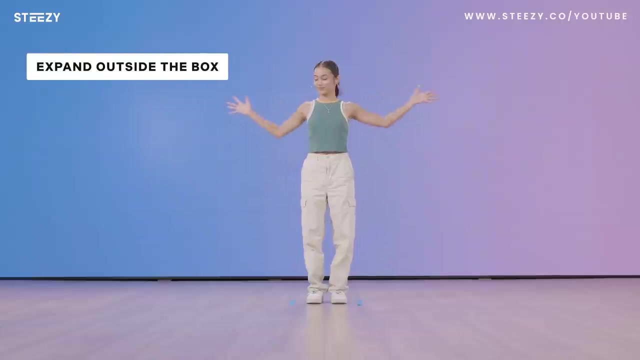 try drawing or taping a box shape on the ground. I recommend painter's tape so it doesn't damage your floors. Your first practice is to expand your arms, legs and even your neck beyond the box by hitting a pose that breaks the box, then closing back in. Repeat that 10 to 20 times. 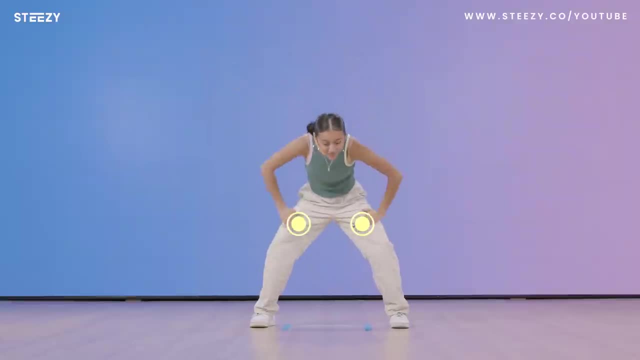 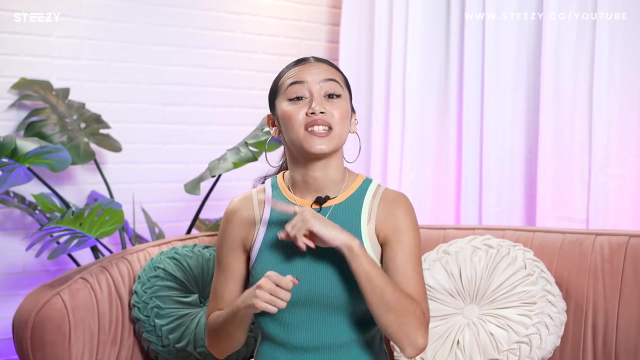 You'll know you're expanding properly if your armpits, thighs and neck can breathe. This expanding and posing might feel cheesy at first, but I promise it will actually make you look much more confident and inviting. Now let's level up this practice by dancing around. 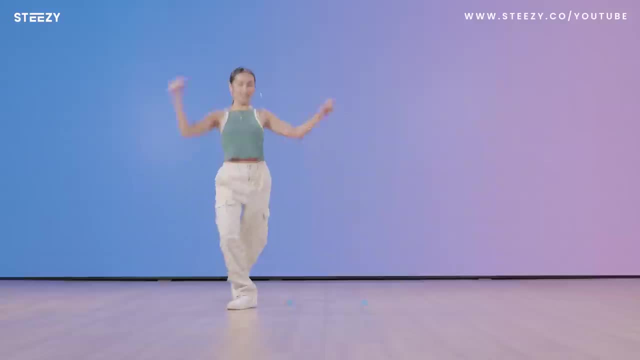 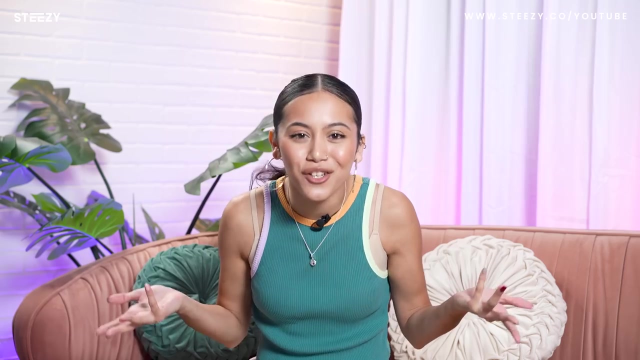 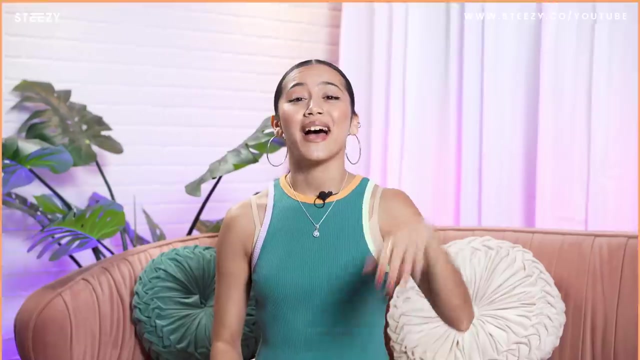 or through the box, without ever stepping in the center. Now look at you go. You're traveling more on the floor, opening up and looking less awkward. Let's keep this energy up and adjust to the next bad habit, Bad habit number two: having a stiff neck. Of course, you don't only want 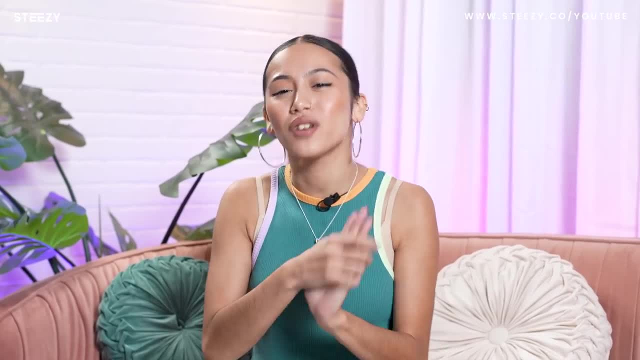 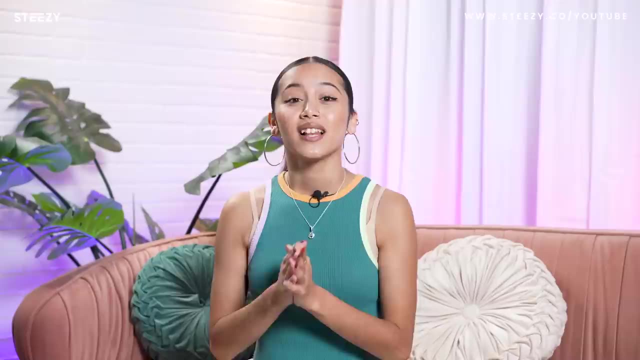 to fix your stiff neck. you want to fix the whole stiff body. But did you know, just by loosing and being more decisive with your neck motion, you can instantly make your dancing look less awkward. Let's go over a few warm ups and stretches to loosen our neck. 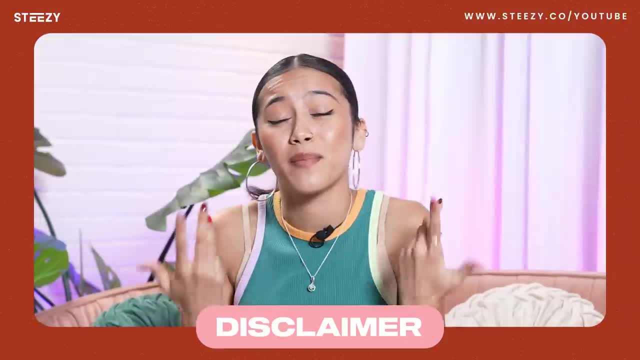 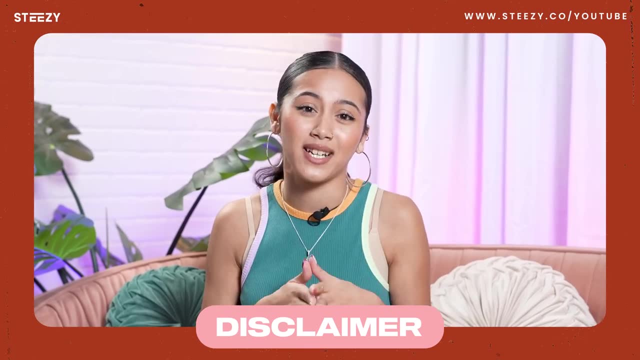 Do keep in mind that I am not a licensed medical professional, So what I am about to say shouldn't be used as a substitute for professional medical advice, diagnosis or treatment, especially if you have neck pains and soreness. Number one: shoulder rolls. 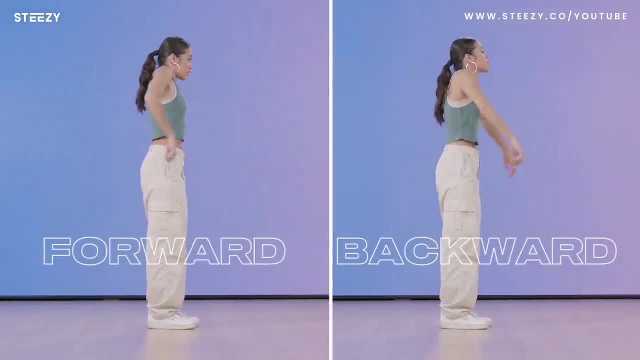 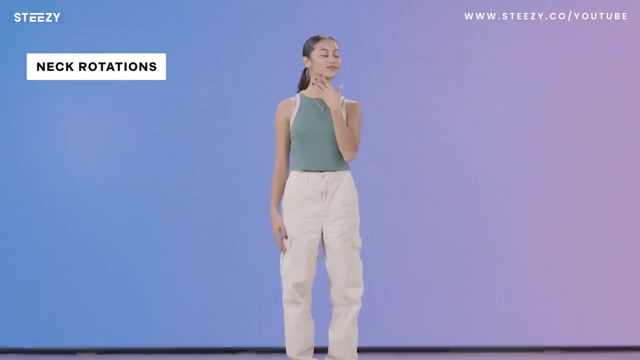 Don't rush these. Roll your shoulders forward eight times and backwards eight times. Number two: neck rotations. Keep your shoulders relaxed. Slowly turn your head to one side as far as you feel a stretch on the opposite side of your neck. Hold for a moment, then slowly go back to where you started and repeat on the other side. 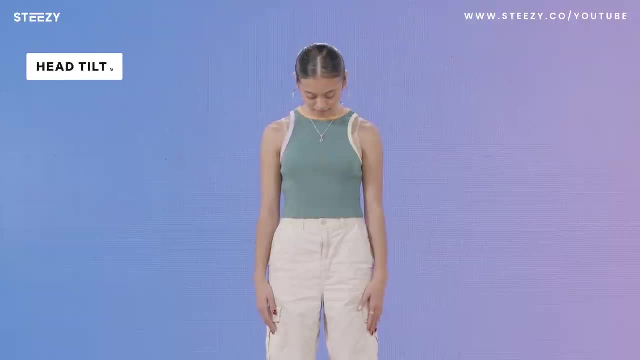 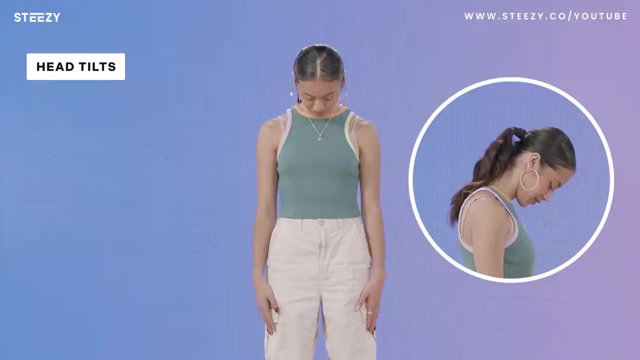 Number three: tilts. Tilt your head down and hold for two seconds. then tilt your head upwards and hold for two seconds. Repeat eight times each side. Number four: neck rolls. Gently tilt your head to the right and hold for four counts. 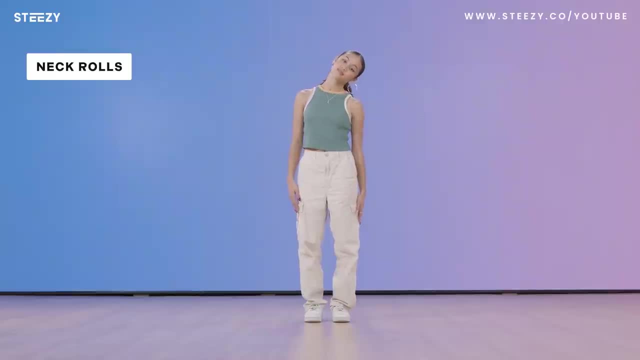 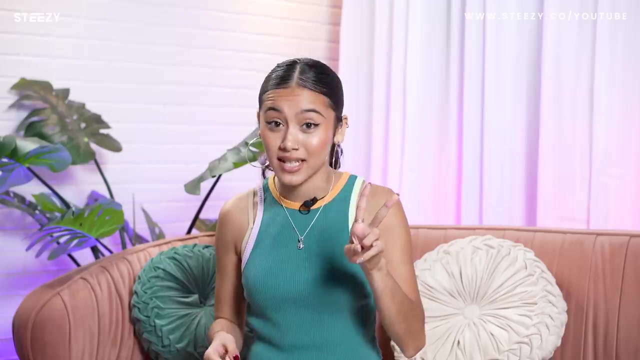 then roll it through the center to the left and hold for another four counts Again. repeat this eight times each side. A good tip is to take nice deep, calm breaths as you're stretching to keep your body fit. You can do two repetitions of all these warm-ups and stretches at a time, twice a day. 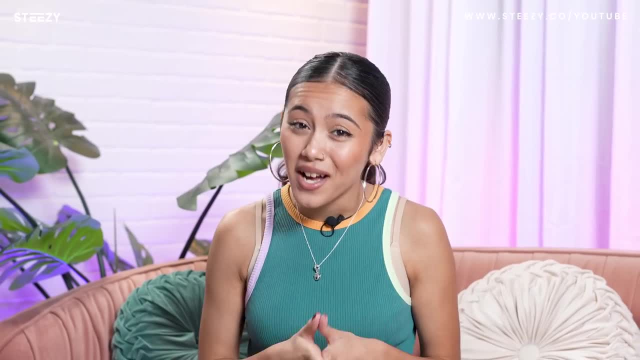 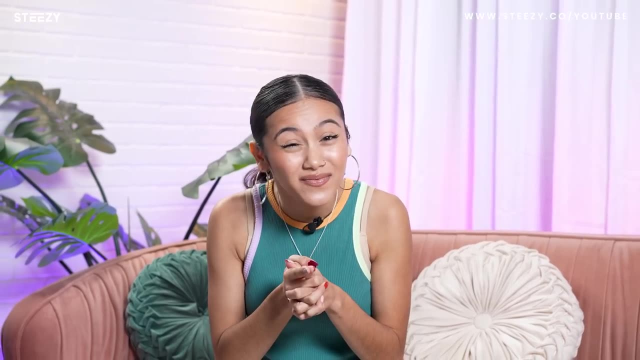 so that's a total of four repetitions in a day. Now that we know how to loosen our neck, how do we show that off when we dance? I have a question: How many directions and ways can we look? I'll give you a moment to think about it. 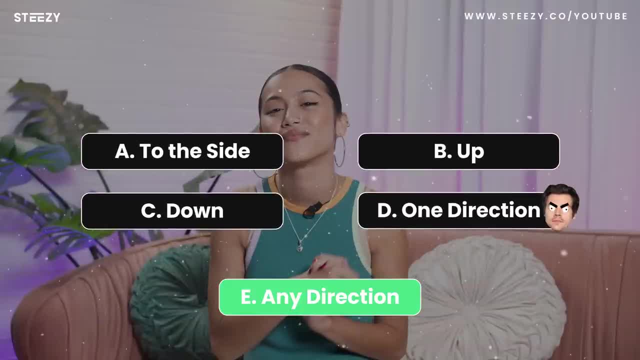 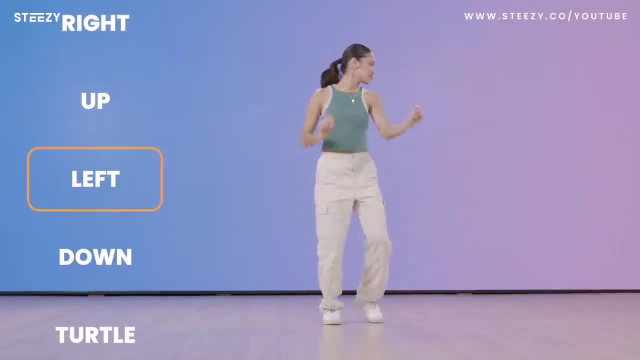 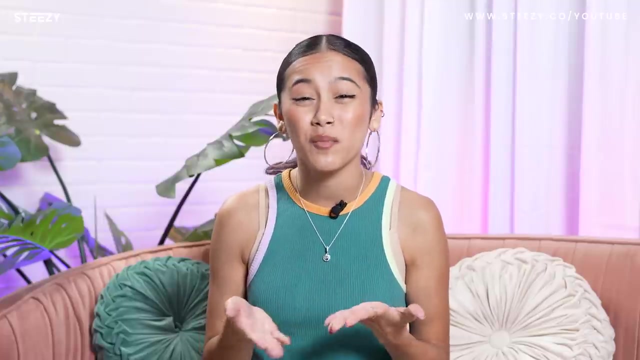 The answer is E pretty much any direction. Turn your head right up, left and right Down, turtleneck, snake, tilt or roll it If you feel like you have a hard time grooving or keeping rhythm in your body. 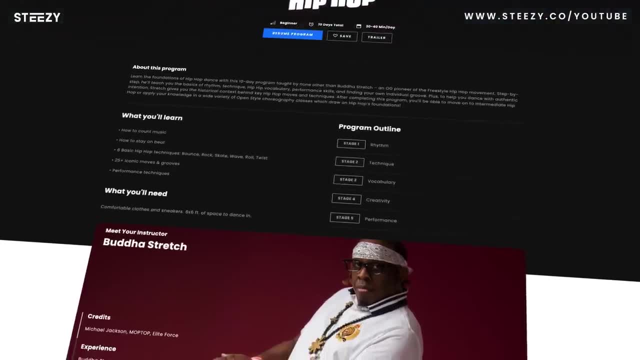 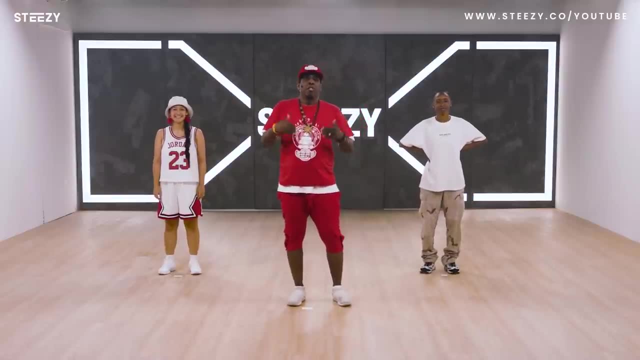 I highly recommend taking Buddha Stretch beginner hip-hop program on STEEZY Studio. The first class in the program is literally about rhythm. Your rhythm is your connection to the beat, to the music, to the cadence. We'll put a link in the description for you. 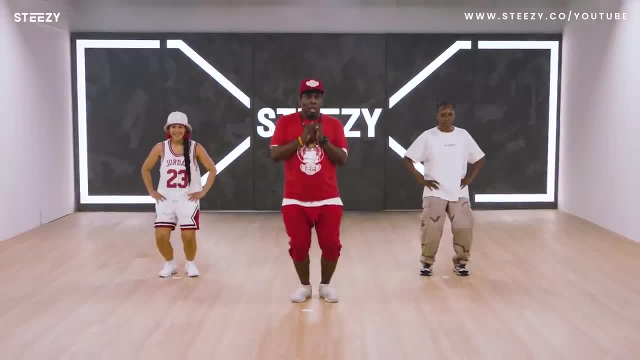 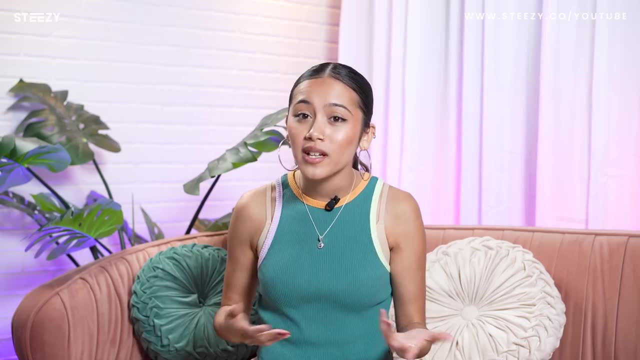 Link in the description for a seven-day free trial of STEEZY Studio so you can give that class a try Now that you've tackled the stiff neck problem and dance outside of your box. you're killing it. We definitely feel more open and relaxed in our bodies. 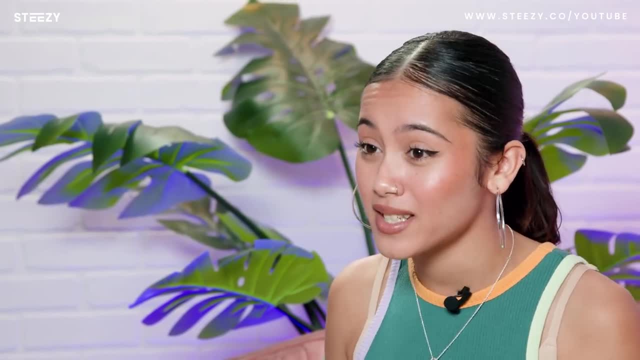 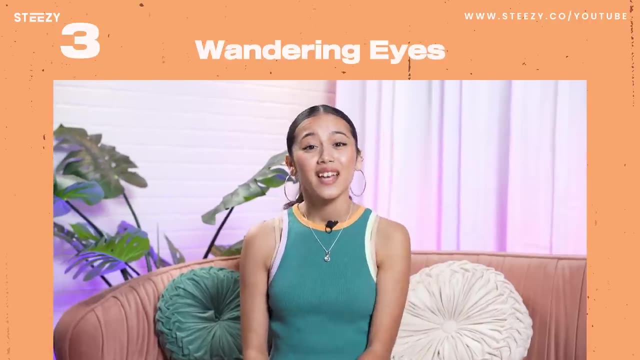 but the best dancers don't only connect with the rhythm and their bodies, they connect with their audience. and you'll have a hard time doing that if you have Bad habit. number three: wandering eyes. This one is easy to miss but so vital in our journey towards tackling our dance awkwardness. 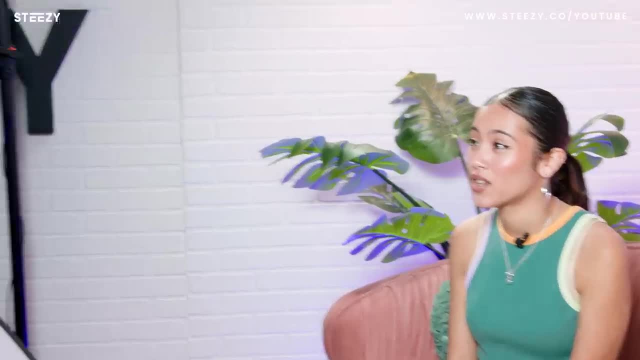 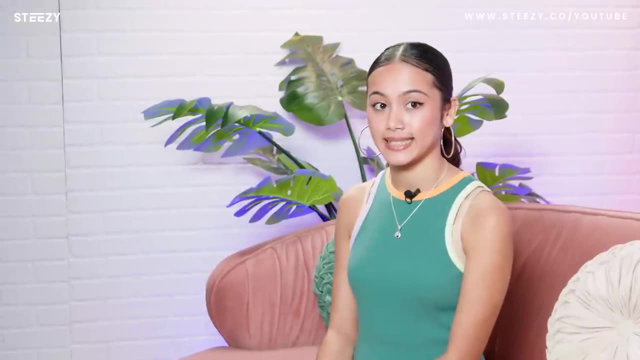 Have you ever talked to somebody and their eyes just drift off from you, Drift off from your eyes for elongated periods of time? This can feel disconnected from the person you're talking to or, in terms of dance, the people you're dancing in front of. 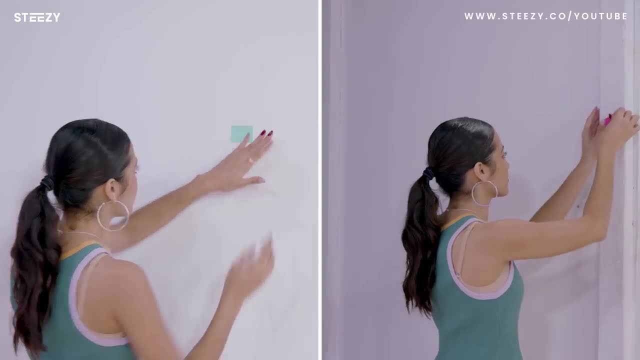 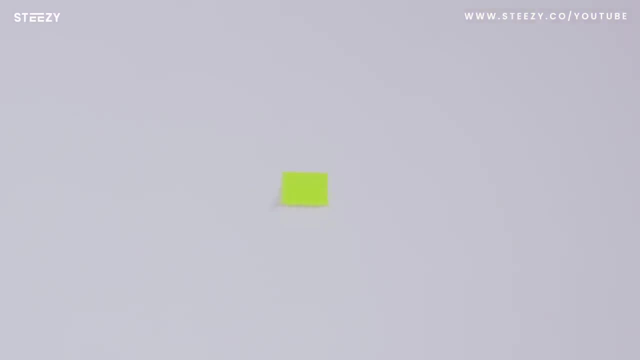 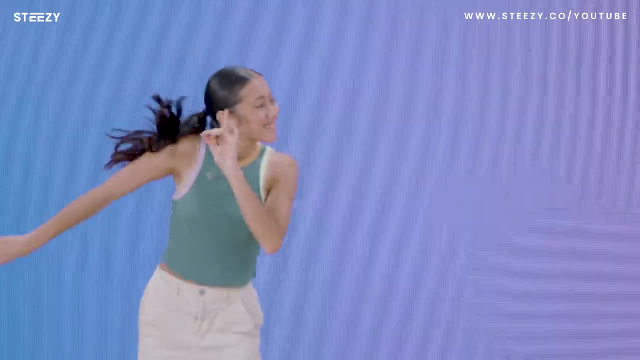 The way my old teacher suggested practicing this was to put sticky notes around the room and we'd have to hold focus on them as we danced. That's when we can complete our dance moves. The level up from that is using people as your focus. 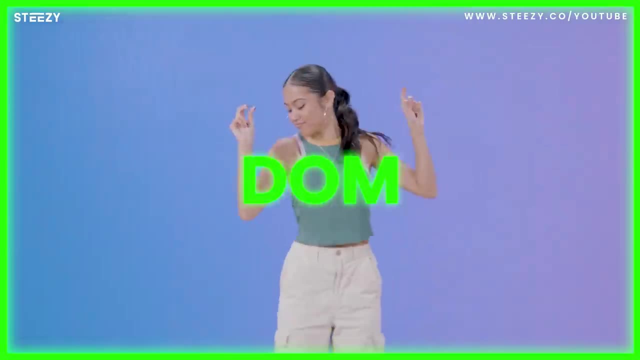 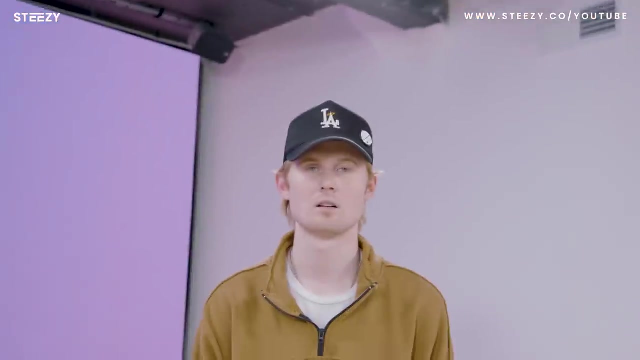 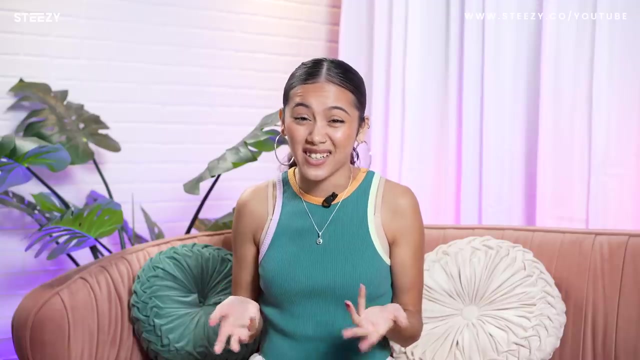 The level up from that is using people as your focus. Dancing with the大家好, Dancing with theซ- Okay, not literally having people stand there and stare at you, but you have to keep in mind that that's kind of how dance circles and performances work. 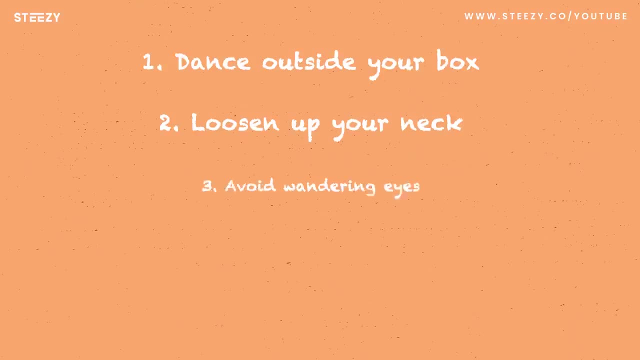 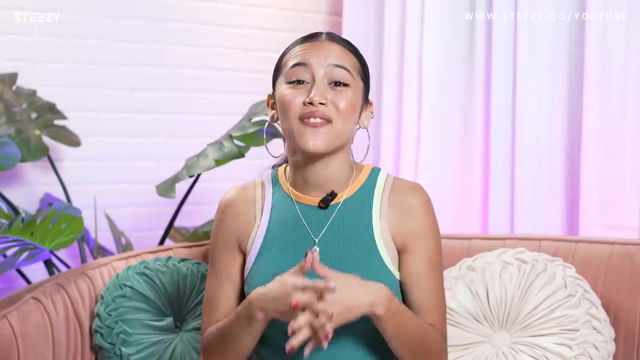 work. a bunch of people watching you dance. as long as your eyes aren't wandering, you're on the right track. just make sure you are confident in where and how you're moving while holding focus, or else you'll have to address bad habit number four: falling off balance. there are three main reasons. 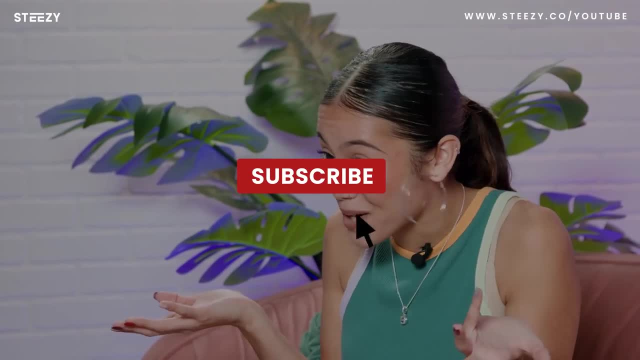 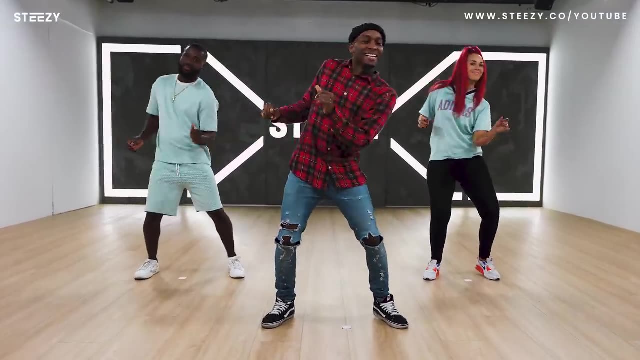 why people fall off balance when dancing. number one: they're not subscribed to the channel. number two: they're not keeping their knees soft. tango elitist mentions this in the first class of the beginner dance hall program on steezy. he tells you to keep soft. first of all, our knees are going to. 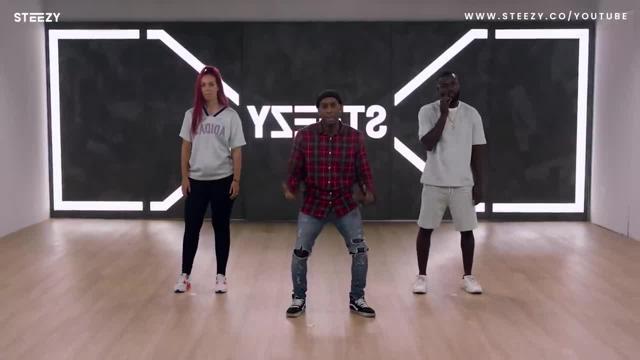 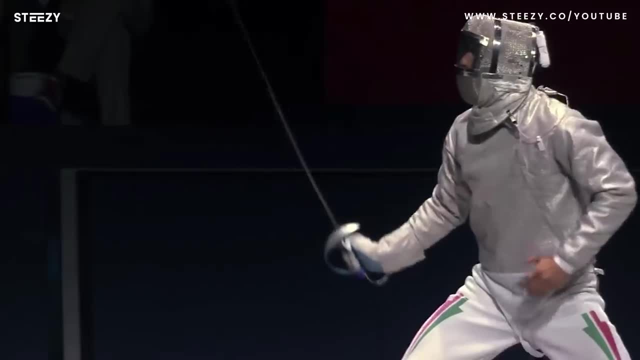 be soft, okay. so with soft knees and we mean they're going to be bent, all right, not crazy bent, you're not going to be down here, but you sure ain't going to be straight up like this. yeah, even in other sports athletes have soft knees because they're always prepared to move, whether it's a 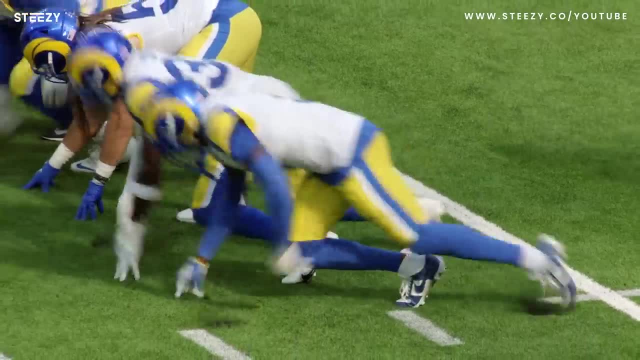 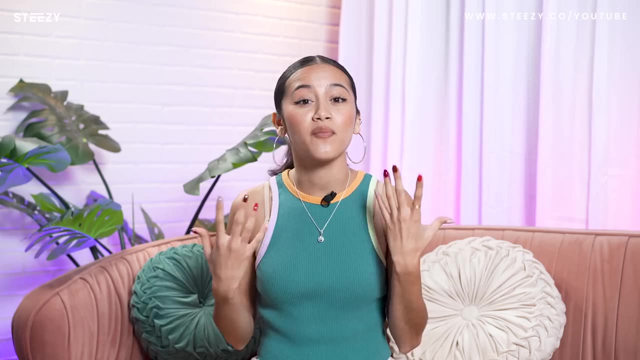 basketball player guarding an opponent, or a football player prepared to sprint. keeping your knees slightly bent also helps lower your center of gravity, giving yourself more stability. a third reason why people fall off balance when dancing is because they have a weak core or simply don't engage their core. 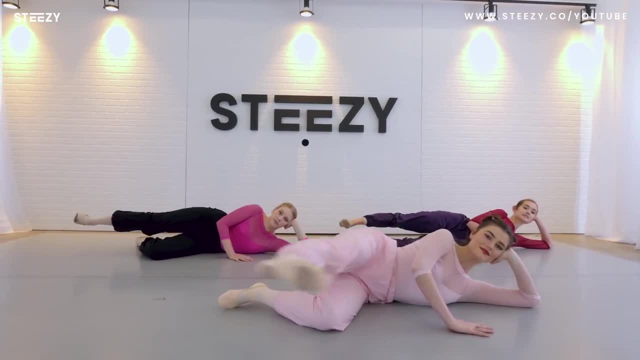 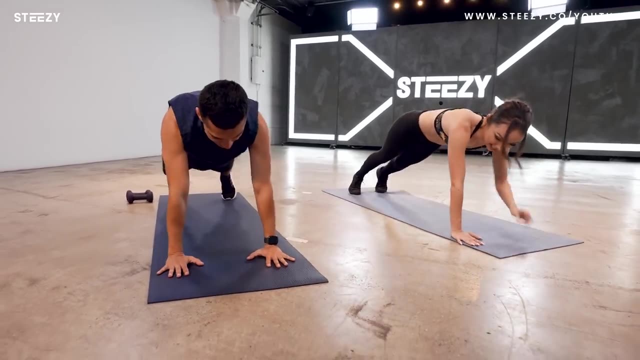 your core, contrary to popular belief, is not just your abs, it's the pelvis, lower back, hips and stomach muscles, and the best first step to engaging these body parts is to work out your core. rachel woods ashiro has a sick 15 minute standing core workout on steezy that she leads us through while 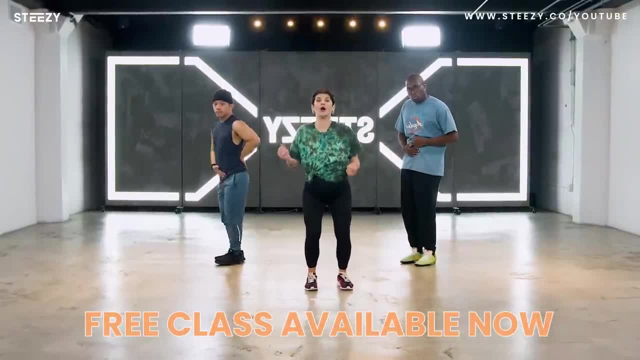 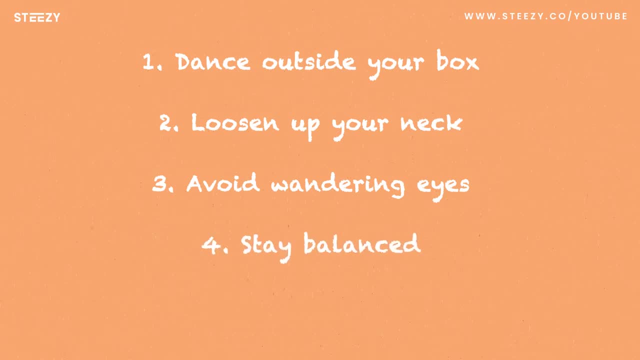 she's pregnant. you know what? just for y'all, we'll drop that video for free on youtube at the same time as this video link is in the description and here at the top. take that class after you finish this video. now that you're more balanced, you can hold focus with your eyes. your neck is loosened. 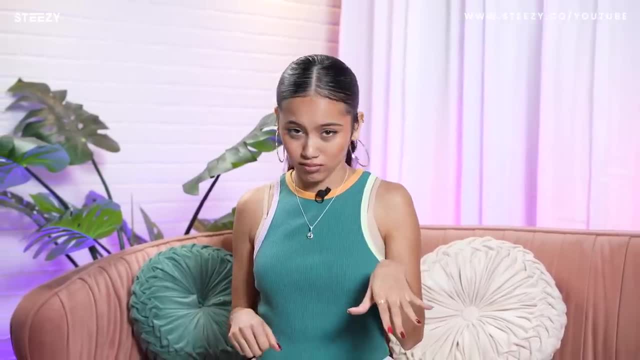 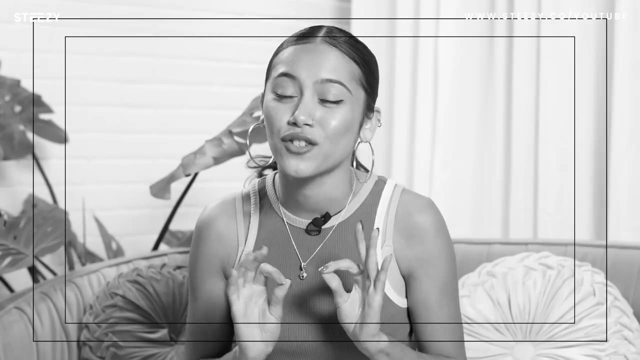 you're out of your box. you're good, right, wrong. bad habit number five: not tracking progress. we mentioned at the beginning of this video that you should record your progress along the way as you practice the steps in this video. this is because one of the most difficult parts of dance isn't the 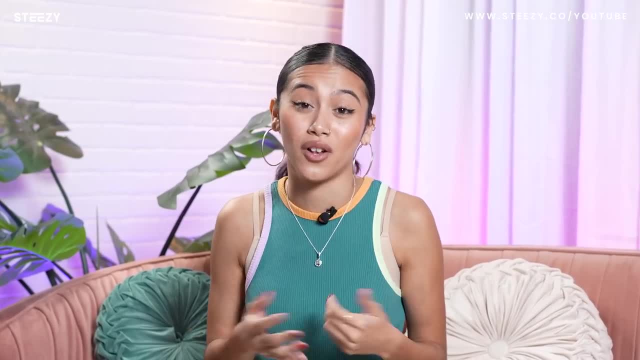 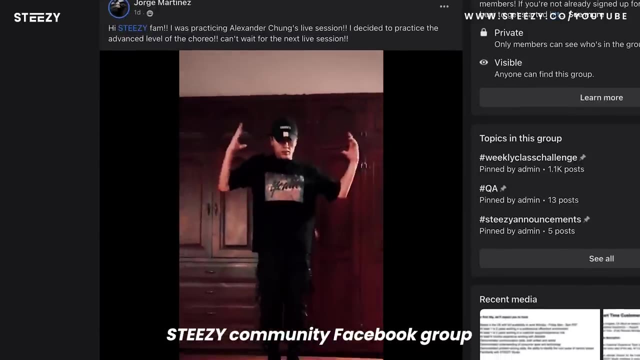 dancing itself, but actually seeing and acknowledging our own growth along the way. so record videos of your dancing and practices and tell the camera what you're about to learn or do and how you're feeling before and after each practice. it's too easy to beat ourselves up when